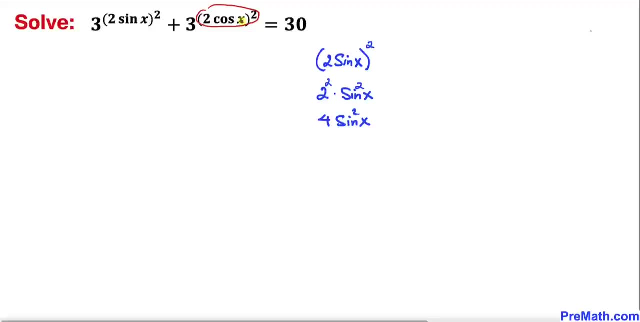 another exponent, 2 cosine of x, whole square. and here I have copied it down and this could be simplified to 4 cosine square of x. So therefore our this equation is simply going to become 3 power. I'm going to replace this by this one, So I can write 4. 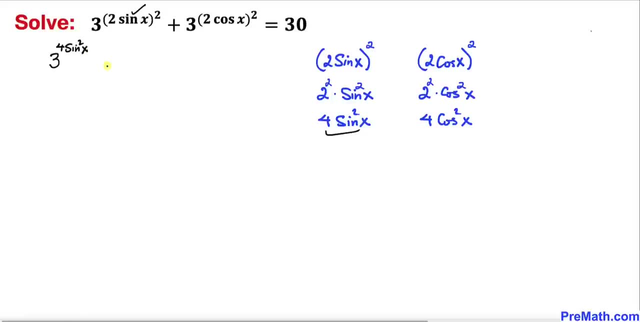 sine square of x and then plus 3 power. I'm going to replace this exponent by this one, So that's going to be a 4 cosine square of x equals to 30 on the right hand side. and now let's edge. Now let's take this power rule. by using this power rule on these exponents, we can write this one: 3. 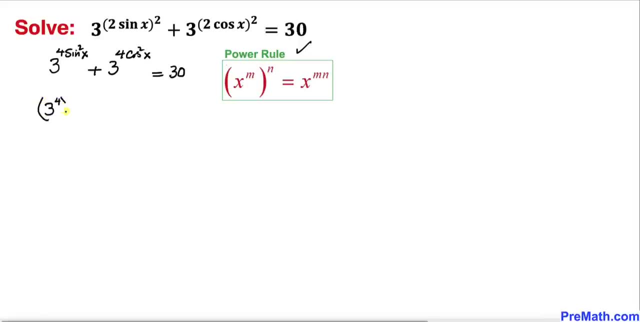 power 4 and then whole power sine square of x plus. likewise I can write this one: 3 power 4, power cosine square of x equals to 30, and now let's focus on this part over here. and 3 power over here as well. and we know that 3 power 4 is equal to 81, so therefore, 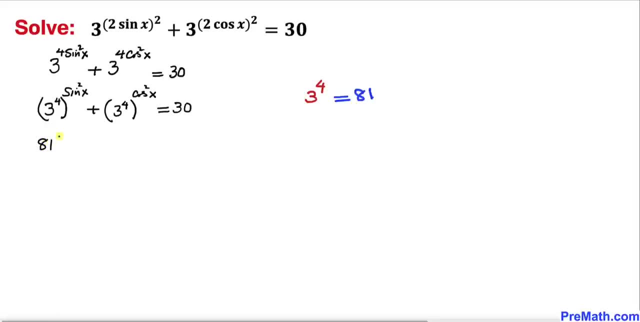 our. this equation is going to become 81 power sine square of x. and now let's recall this famous trigonometric identity: sine square of x plus cosine square of x is always equal to 1. now let's move this sine square of x on the right hand side, so that is going to give us cosine square of x. 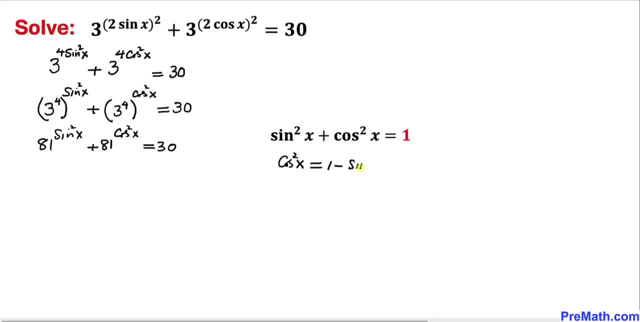 equal to 1 minus sine square of x. now i'm going to replace this cosine square of x by this part: 1 minus sine square of x. therefore, our this equation is going to become 81 sine square of x plus 81 power. i'm going to replace this one by 1 minus sine square of x. 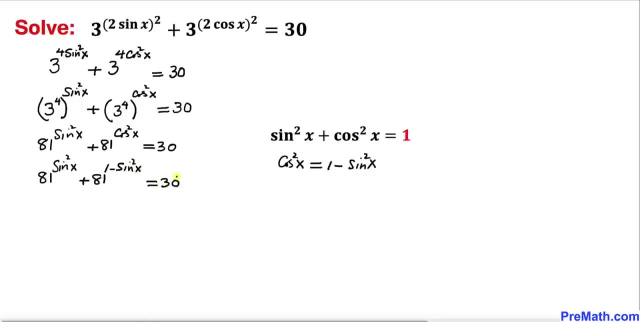 equals to 30 on the right hand side. now let's focus on this term: 81 power 1 minus sine square of x. and here i have copied it down and let's go ahead and simplify it now. if we use the rules of exponent, we can write 81 power 1 times 81 power negative sine square of. 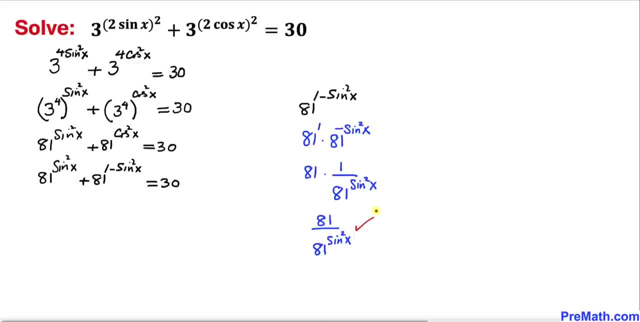 x and whatever. 1 times h is equal to 1 minus sine square of the integral of xi, plus unaware of 1 times h of 8, and therefore that is not 핫 수oof蛋. so therefore this has been simplified to this, so therefore this equation could be written as 81 power sine square of x. plus 81, divided by eight eem, one power sine square of x equals to 30. now we want to make our job easier by doing the substitution. let me look at this one. i'm этойlerhene: hannadi hannadi, hannadi hannadi. 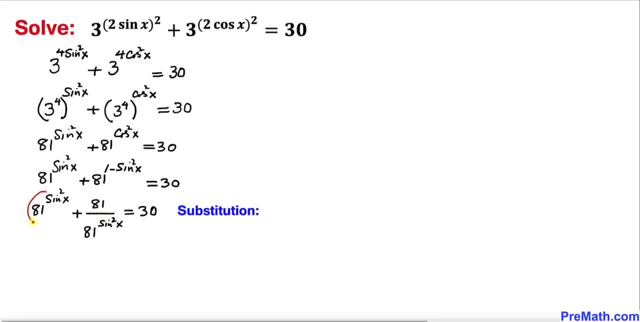 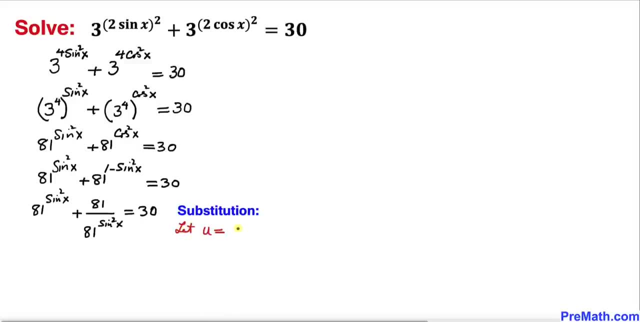 let u equals to 81, power sine square of x. so therefore our this equation is going to become: u plus 81, divided by u equals to 30. let me go ahead and remove this fraction by multiplying by u across the board. so we are going to a u times u is going to give us u square plus this u and u. 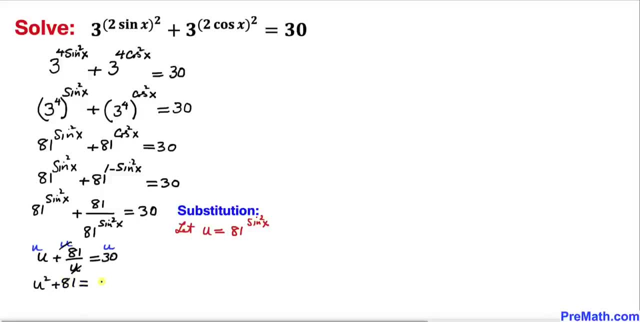 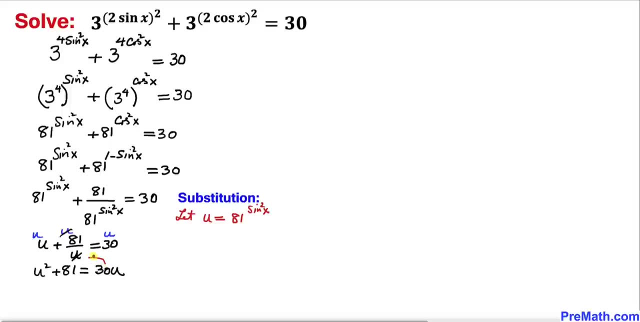 is gone. we got 81 equals to 30? u on the right hand side, and now let's go ahead and move everything to the left hand side and put in a descending order, and here our equation is going to become: u square minus 30, u plus 81 equals to 0, and now we are going to solve this. 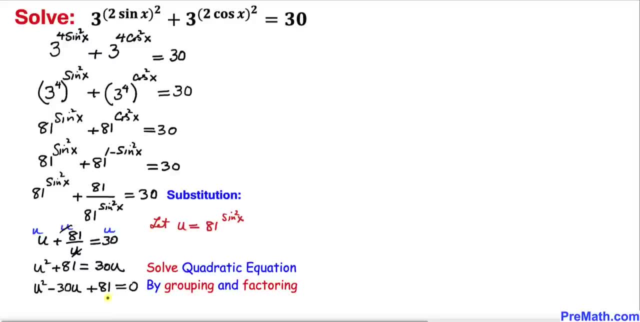 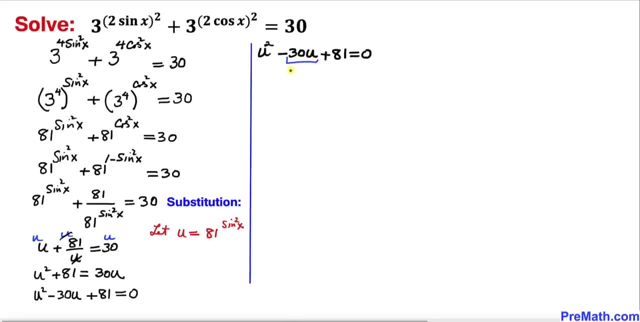 given quadratic equation by grouping and factoring. and now let's focus on this part of this quadratic equation: negative 30 u. let me go ahead and tweak it. i can write this one as negative: 3 u minus 27 u. and here we can see that u is in common between first two terms and over here. 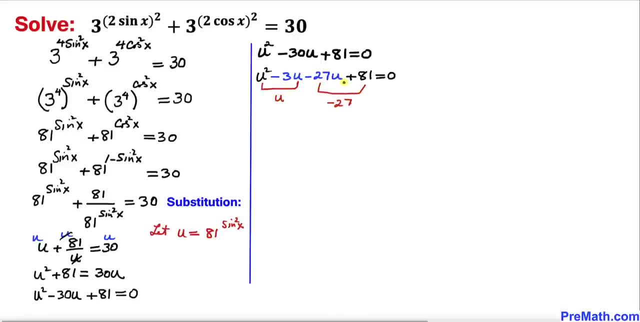 negative. 27 is common between these last two terms, so therefore we can write u outside: u minus 3 and minus 27 is common. over here we can write u minus 3 as well. equals to 0, and now we can see u minus 3 and u minus 3. they are in common. so we can factor that u minus 3 outside and we get 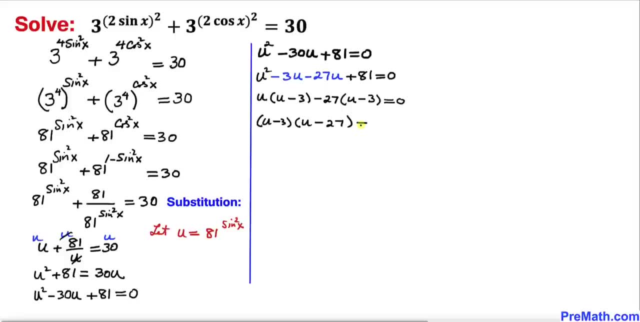 u minus 27 equal to 0. let's go ahead and separate them so i can write u minus 3 equal to 0, and this side is going to be u minus 27 equal to 0. so that means we're going to have u equals to positive 3 and on this side we are going to have u equals to positive 27, but then 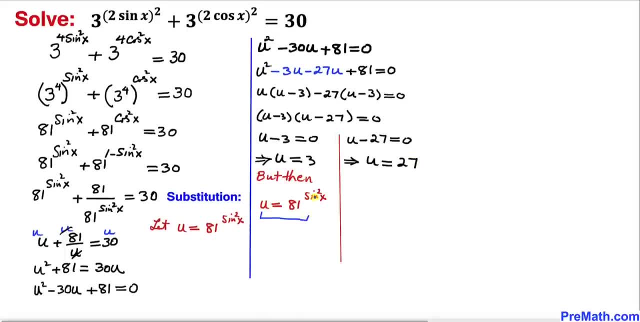 we know that u equals to 81 power sine square of x, so therefore we can write: 81 power sine square of x equals to 3. and now let's focus on this base. 81 know that 81 could be written as 3 power 4, so therefore I'm going to replace this 81 by 3 power. 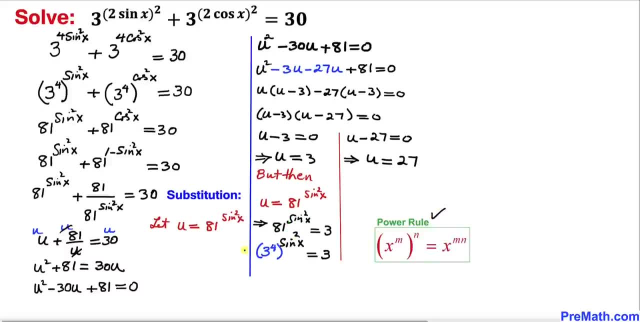 4. Now let's go ahead and apply this power rule on the left hand side. so this could be written as 3 power 4. sine square of x equals to this. 3 could be written as 3 power 1, and now we can see that. 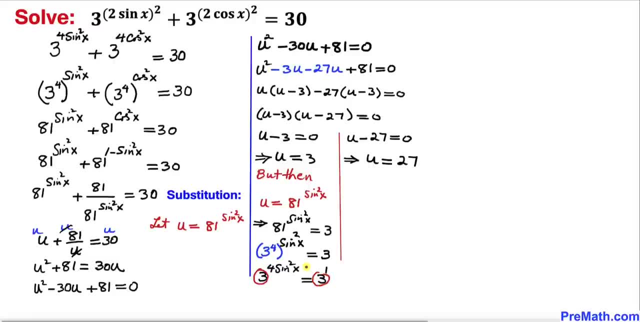 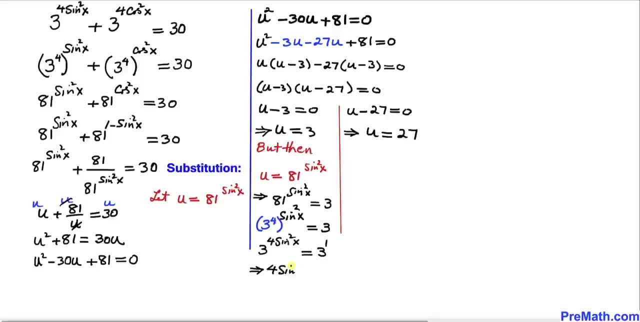 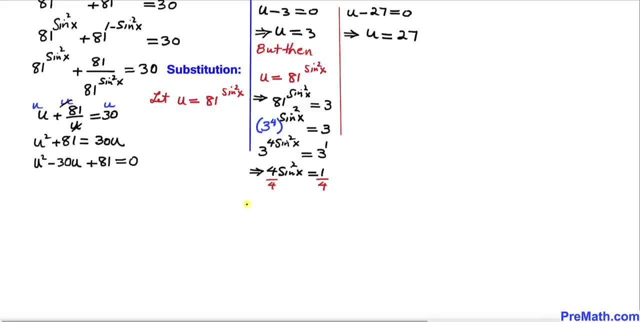 our bases are same on both side, so therefore we can equate our exponents. so therefore we can write 4: sine square of x equals to 1, and now let's go ahead and divide both side by 4, so we are going to get sine square of x equals to 1 over 4.. Let's go ahead and take the square root on both sides. 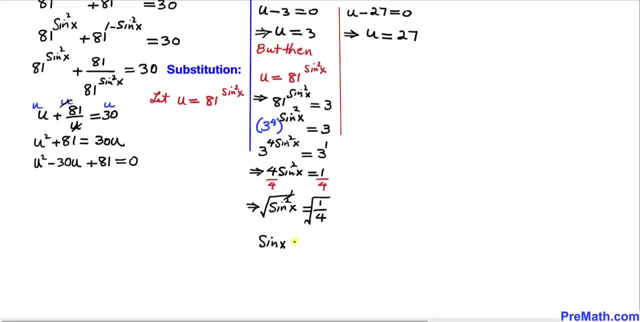 so we got: sine of x turns out to be positive or negative, 1 over 2, and now let's focus on this equation. on the right hand side, u equals to 27, but we know that u equals to 81, power sine square of x. so therefore we can write 81: power sine square of x equals to 27, and now we know that this 81. 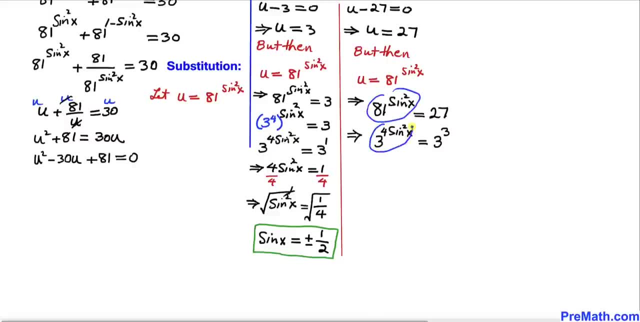 power sine square of x equals to 27.. So let's go ahead and write 81: power sine square of x equals to 3, and now we can see that our bases are same on both side. so therefore we can equate the exponents. so therefore we can write: 4 sine square of x equals to 3.. Now let's divide both side by 4. 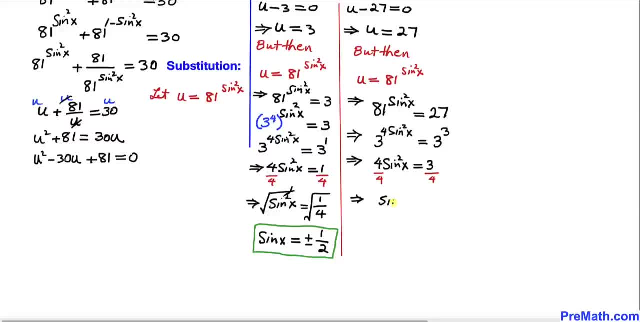 so, therefore, we are going to have a sine square of x equal to 3 divided by 4.. Now let's go ahead and take the square root on both sides to undo this square. so we got sine of x equal to positive or negative square root of 3 divided by 2.. Therefore, we got these: 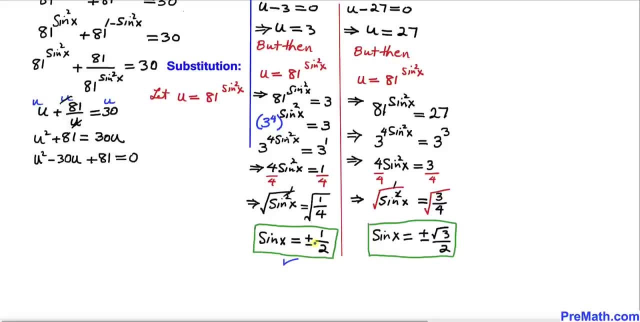 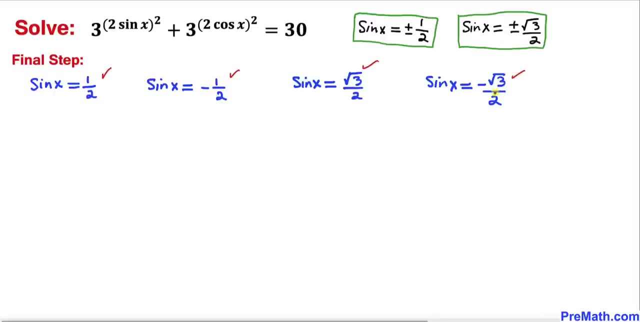 values. first one is sine of x: equals to positive or negative 1 over 2. and the second one is positive square root of 3 divided by 2. and here's our final step. we got all these four values of sine of X, as we found out in our previous steps and we know that if 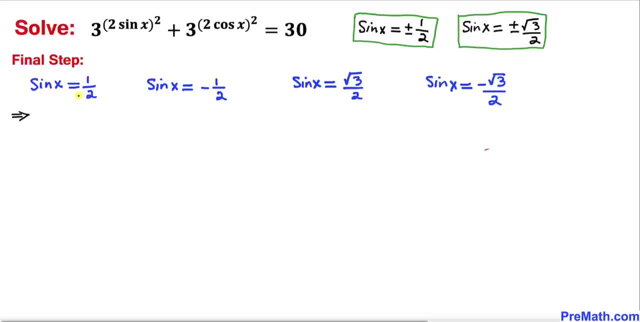 sine of X equals to 1 over 2, then we can use a scientific calculators are the trig tables. our X value is going to be 30 degrees, and if sine of X is negative- 1 over 2- then our X value is going to be 210 degrees, and likewise in this case. 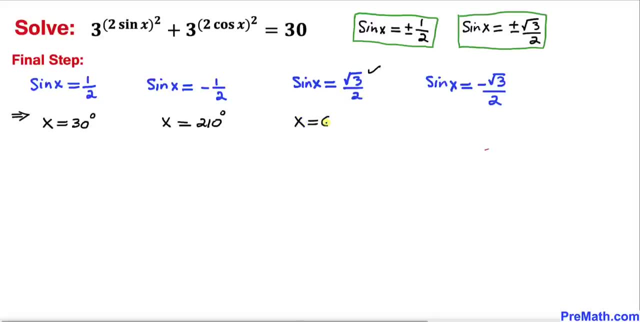 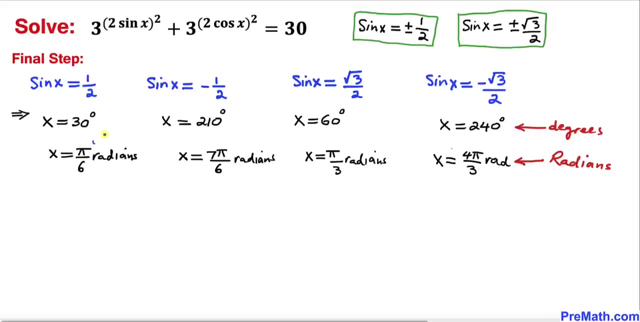 is going to be X equals to 60 degrees and finally, for this one, X equal to 240 degrees, and if we write them in terms of radians, so this is going to be a pi over 6 radians. this is going to be a pi over 6 radians, this is going to be a pi over 3 radians and finally, this is: 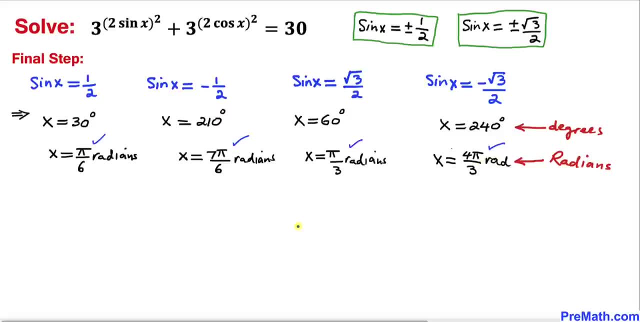 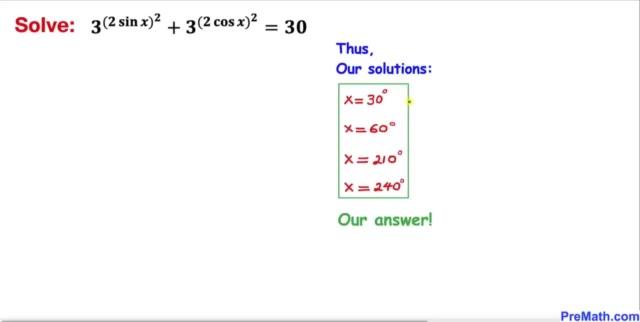 going to be 4 pi over 3 radians. and finally, if you have any question, how to convert from degrees to radians and vice versa, I have already uploaded video on this topic. please check it out. in the description below and here are four solution in terms of degrees and here are our solution in terms of radians. 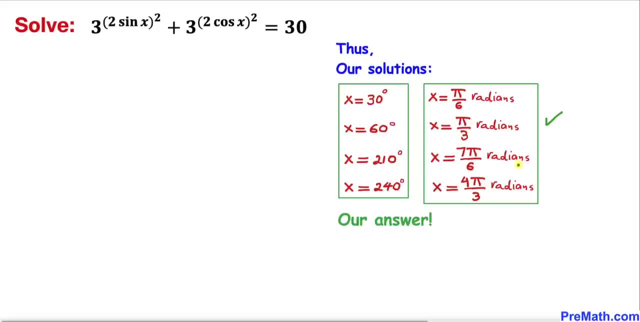 thanks for watching and please don't forget to subscribe to my channel for more exciting videos. bye. 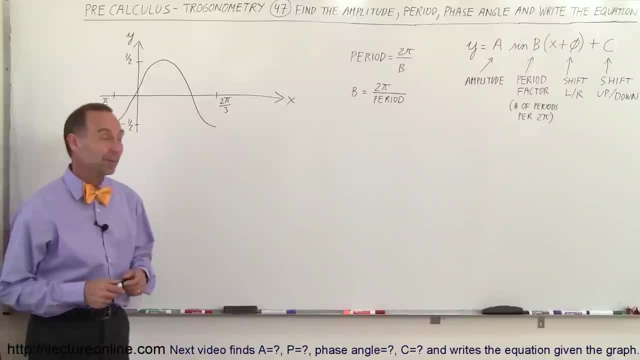 Welcome to Electron Online. and here's a little bit more challenging of a problem. Again, we have the graph, We're supposed to write the equation. We're also supposed to find the amplitude, the period and the phase angle. Let's see here. The amplitude is fairly straightforward. 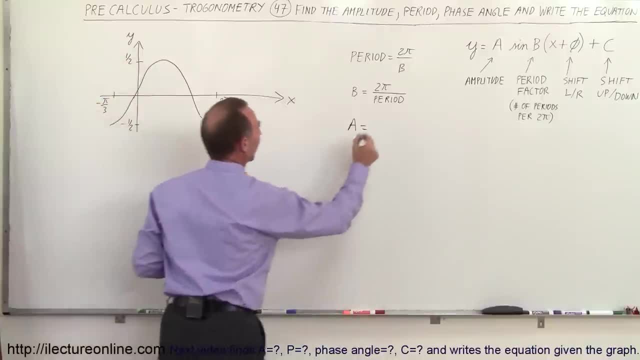 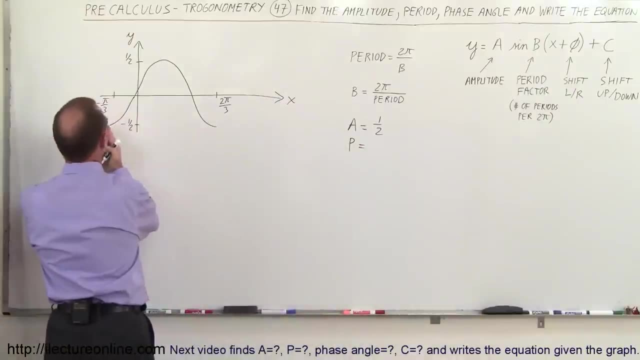 We can see clearly that it goes from plus 1 half to minus 1 half, so the amplitude is 1 half The period. let's see here. we can see that it starts at minus pi over 3 and goes to plus 2 pi over 3.. 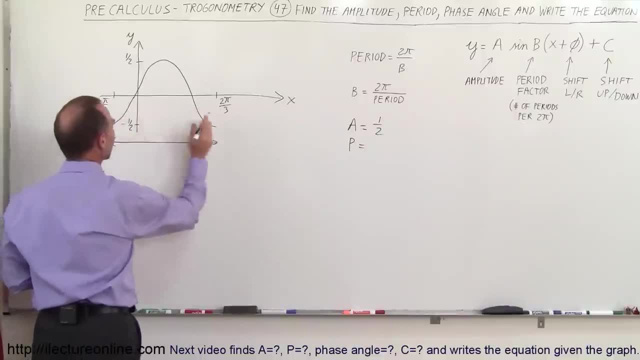 So the whole distance from the beginning to the end of the period is a complete pi. So pi is equal to 2, pi over 3, minus a, minus pi over 3, which is equal to pi. So the period is pi all right. 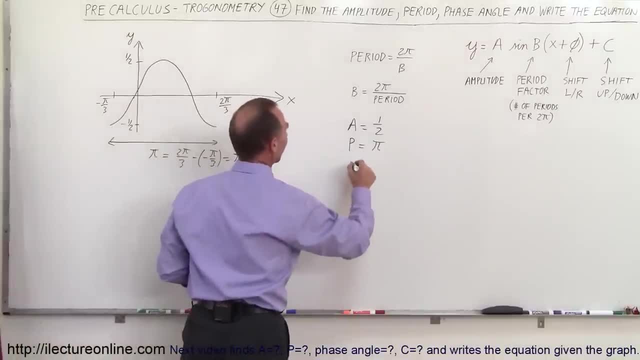 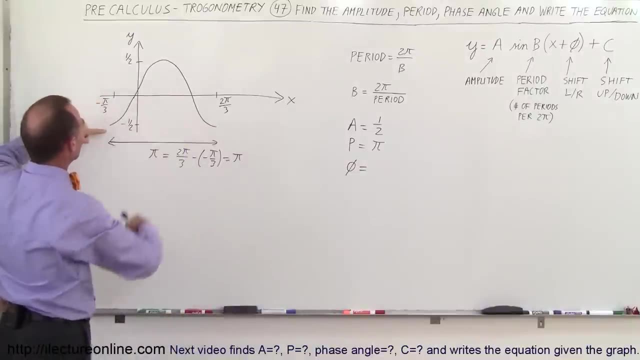 And what else do we have? The period is pi and the phase angle. well, that depends how you want to look at it. What I'm going to do here is: it looks like the function is kind of flipped over. Notice that it starts at the minus maximum amplitude. 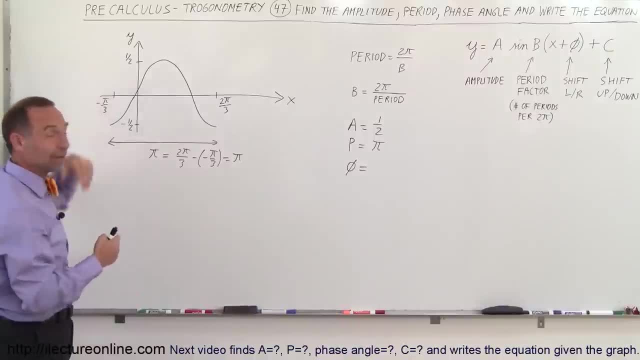 It starts at the positive maximum amplitude. So if this was over here, it would definitely be a cosine function. But we know that the negative in front of the cosine function flips the whole function around. So I'm going to do that. I'm going to put a negative in front of the cosine and then we can see that it's shifted to the left by pi over 3.. 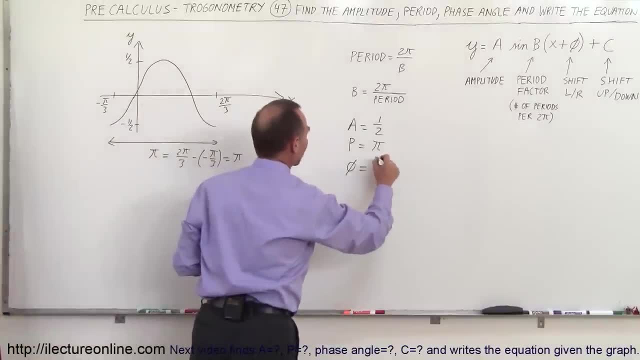 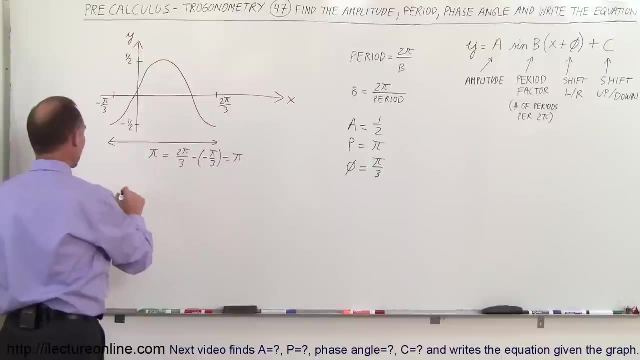 So therefore that will be the phase angle. So the phase angle will be pi over 3, and we know that it's shifted to the left, so we're going to have to add the phase angle plus pi over 3.. So the function then becomes y.